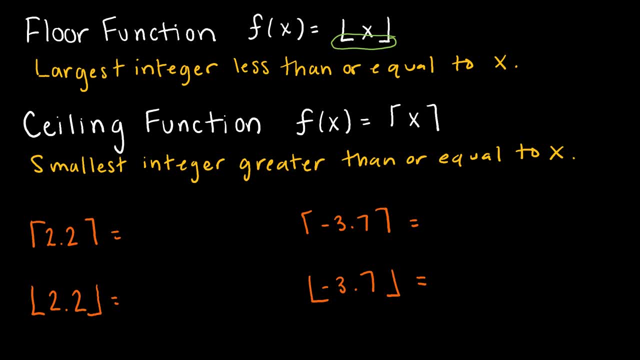 a floor And the ceiling function is similar, but asks us to round up to the nearest integer greater than or equal to x. So let's take a look at an example. I've got 2.2, and if I'm thinking about 2.2 on a number line, then I'm thinking about 2, and then 3, and 2.2 is right around. 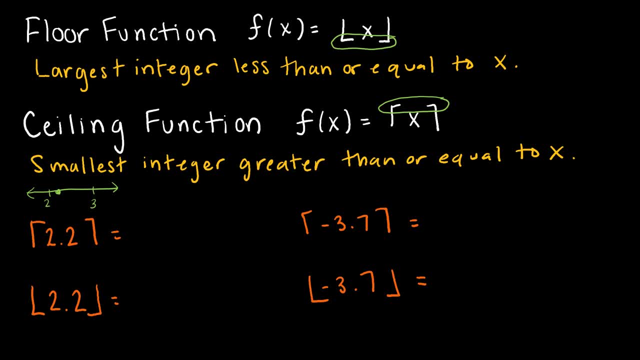 somewhere in there And if I'm rounding or if I'm using the ceiling function, the ceiling function says round up to the next integer and the floor function says round down to the next integer. Same thing happens for my negative 3.7, but just be careful how you put these numbers on the number line, Remember. 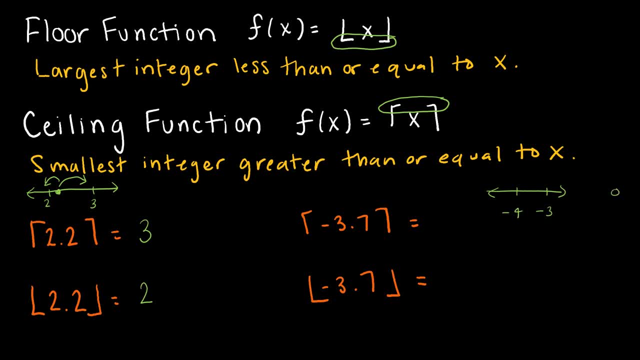 zero is over here somewhere, This would be negative 3,, this would be negative 4, and negative 3.7 somewhere in here. And then if I'm rounding up for my ceiling function, I end up at negative 3.. If I'm rounding down to my floor function, I end up at negative 4.. 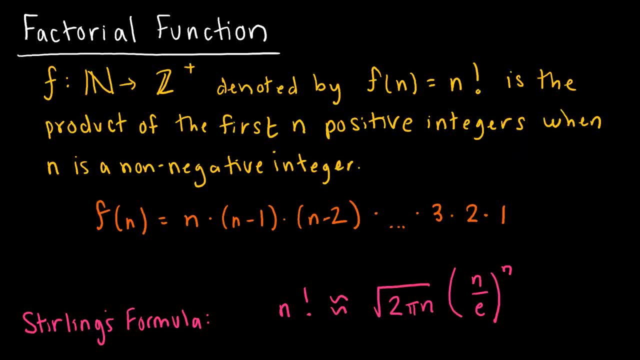 So just be very careful with your negatives, And I am certain, absolutely certain, that you have had the factorial function before. Factorial function is essentially denoted by f of n equals n, that's the exclamation point, which means factorial, And it is the product of the first n positive. 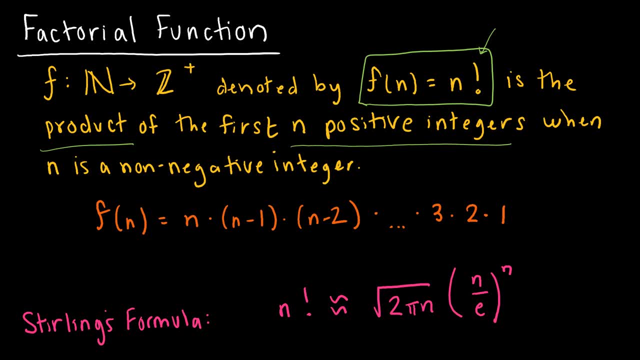 integers when n is a non-negative integer. So I give you an f of n here, but let's say f of 4, I would take 4 times 3 times 2 times 1.. That would be my factorial function: 4 times 3 times 2 times 1.. So again, symbolically, it's n, n minus 1, n minus 2, all the way down. 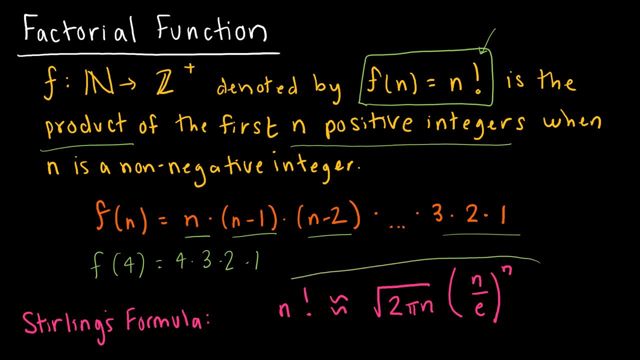 until you get to one. Stirling's formula is fantastic. We're not going to use it a ton right now, but this is a way because that factorial function gets a very large very quickly. this is an approximation that we can find of the product of the numbers of n factorial. 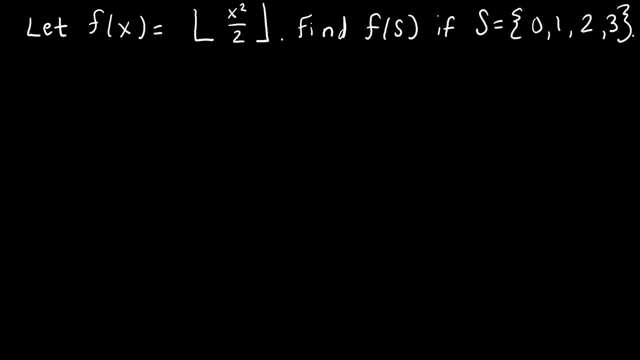 Here's just one more example for you to try. Our function is the floor function of x squared divided by 2, and we're trying to find f of s for the set of s which includes 0,, 1,, 2, and 3.. So 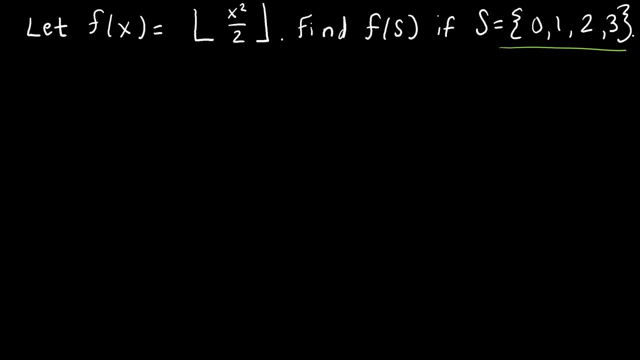 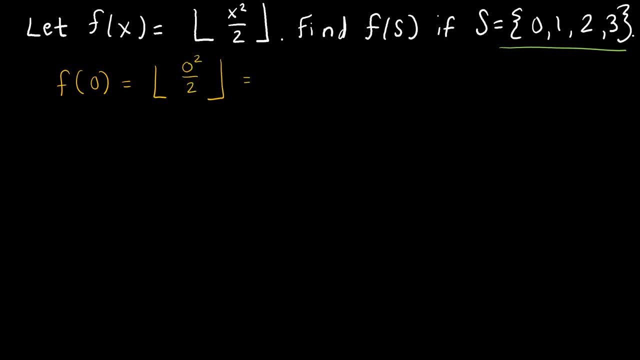 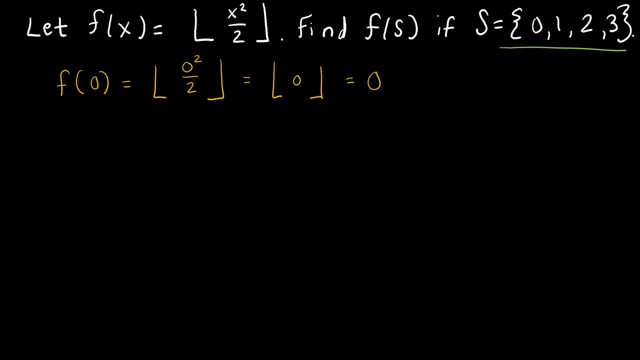 0 would of course be 0.. If I'm looking at f of 1,, f of 1 would be 1 squared over 2, and the floor function, 1 squared, is 1.. 1 divided by 2, that just gives me 1 half. So what is the floor function of? 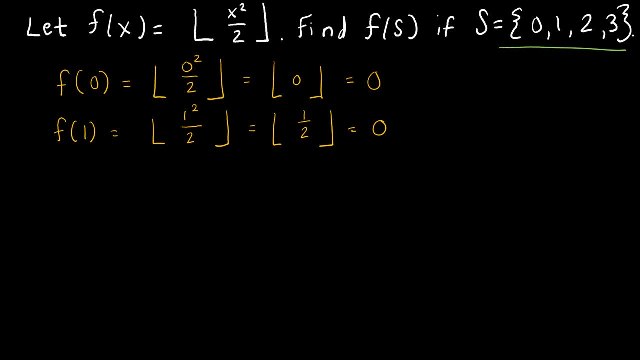 1 half, That is, 1 squared over 2, and the floor function of 1 squared is 1 squared over 2.. So also 0.. Let's do f of 2.. f of 2 is the floor function of 2 squared over 2.. Whoops, Floor. 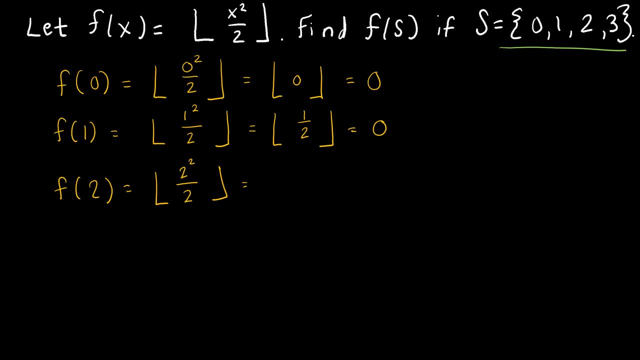 function of 2 squared over 2,, which is 2 squared, is 4 divided by 2, and the floor function of 2,, of course, gives me 2.. And my last one, f of 3, tells me the floor of 3 squared over 2,. 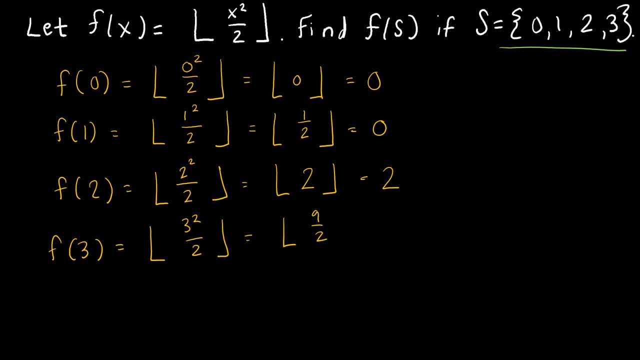 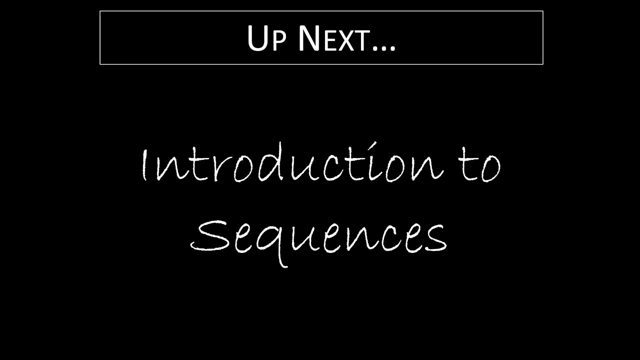 which is the floor of 9 over 2, and the floor of 9 over 2,, which is basically 4.5,, is 4.. So these would be my solutions: 0,, 0,, 2,, 4.. Up next, we are going to switch gears and talk. 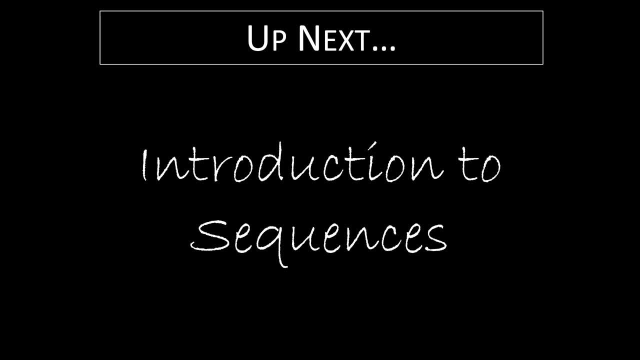 a little bit about sequence, So it's an introduction to sequences.